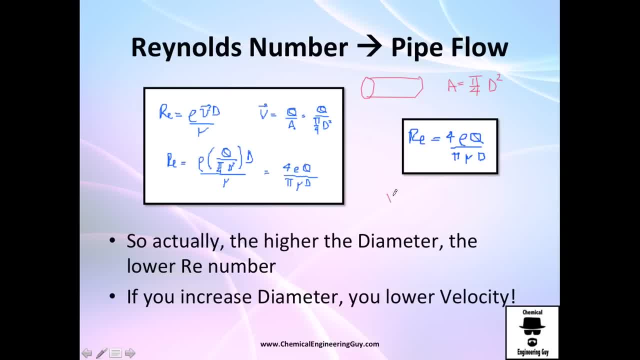 say the diameter we're doing, the area or many times we are given the velocity instead of the volumetric flow rate. so how to relate this velocity with respect to this right here? well, just to this. right here is the Q volumetric flow rate, the area as I. 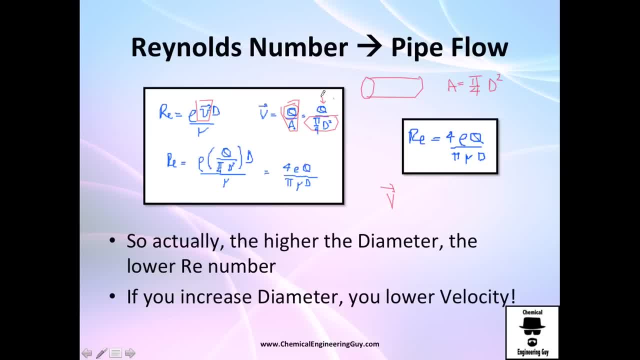 told you before is right here. so plug this value right here in the velocity, in the Reynolds number. so density times velocity, which right now is Q divided by P, divided by 4 times this diameter, square power. don't forget this diameter and the viscosity right here. so arranging and calculating and simplifying, you get this. 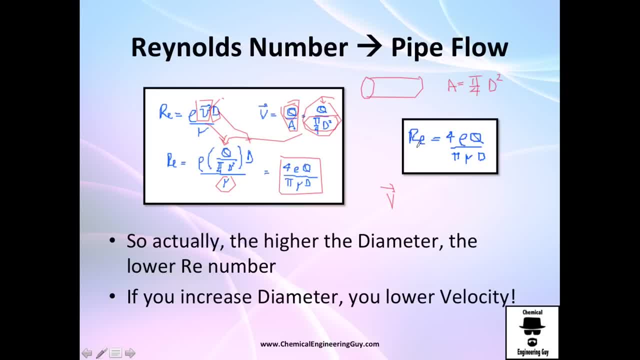 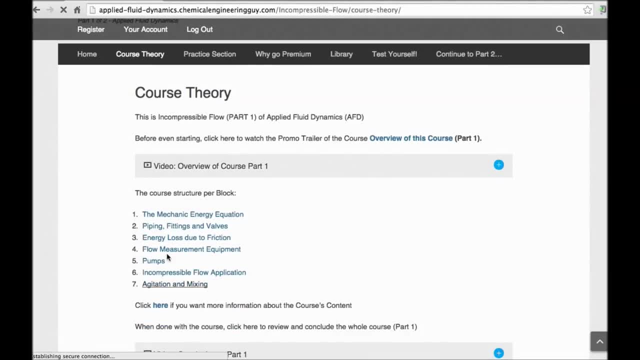 value right here, which is the Reynolds number, when you are given the volumetric flow rate instead of velocity. so instead of you can always check out the course content here. so, for instance, if you want to check out how to measure some flow rate in piping, we got. 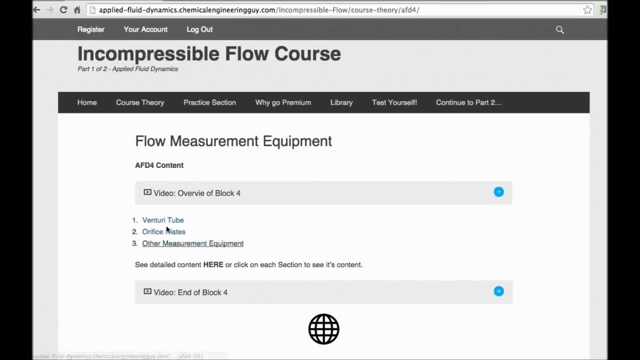 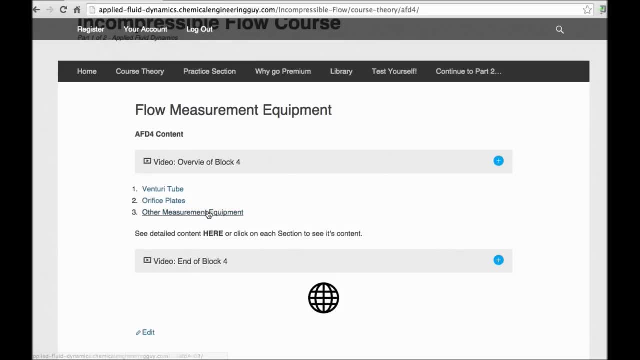 this block, number 4, which is called flow measurement equipment. we essentially have the Venturi tube, the orifice plates, which have essentially the same principle, which is the mechanical learning equation, and learn about other measurement equipment because nowadays we have plenty of other devices that will help us to measure the flow rate in a pipe. having the 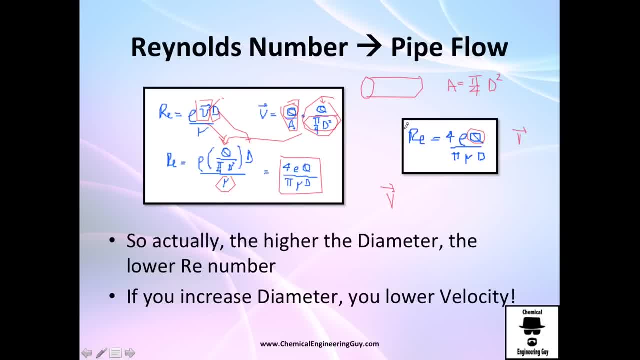 volumetric flow rate and calculating the velocity. we can go and check out directly with this formula. this is valid only on these circular cylindrical pipe. so what you were actually thinking in the Reynolds number, as the diameter increases, what you will tell me. well, a diameter increases, Reynolds. 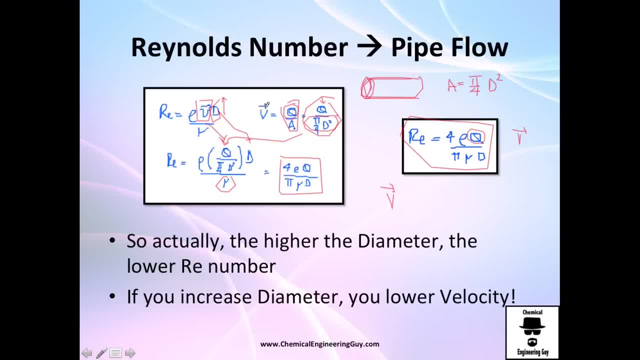 number increases? well, actually not, because velocity decreases with the power of 2. so let's say 10 goes and increases to 20, you will say, wow, we have an increase of 2 times the diameter. so I will expect a Reynolds number twice as big. but actually, if you were to, 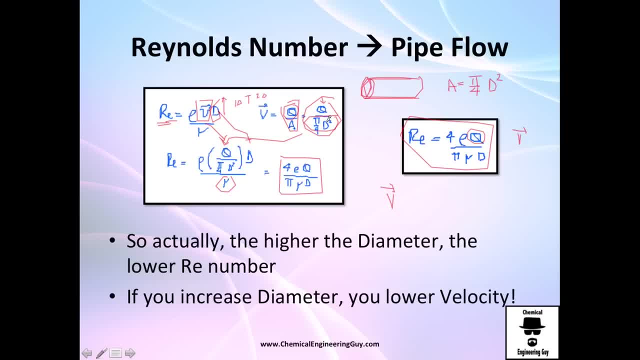 calculate the velocity. the velocity will go four times because will be twice to the second. power will be four times that and they will cancel each other and you will see that actually the Reynolds number is decreasing. so by definition, in a pipe with constant diameter, if you increase. 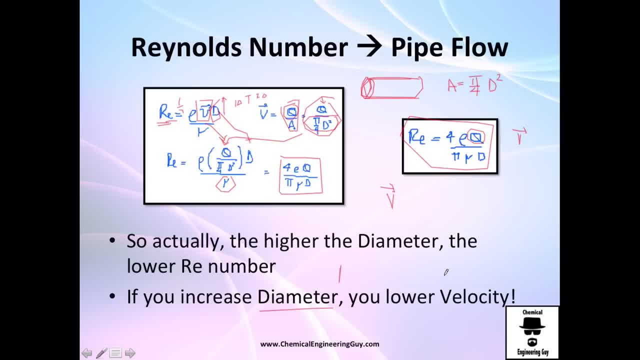 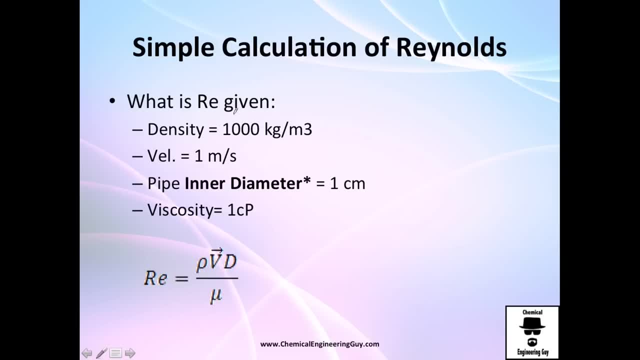 the diameter, you will lower the velocity, which will lower the Reynolds number. let's make this little example: what is the Reynolds number given the density, velocity and pipe inner diameter? so this is very important, guys, because we are talking about the flow and the flow is carried only on this internal, say, area. so we don't want to go out so this. 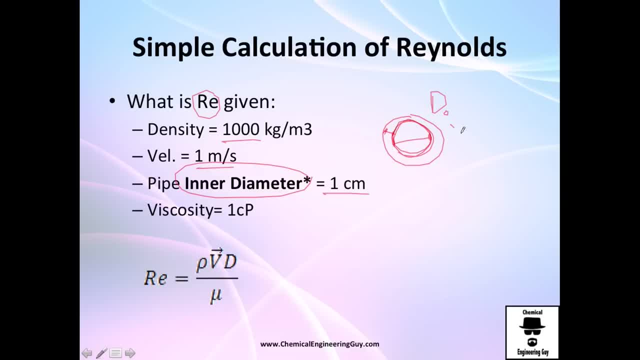 is not. they give you the outside diameter. it won't work because you are, the fluid is not here, so ignore that option. you always need the internal or inner diameter, and let's do it. Reynolds equals this right here and it's very easy. you just need to change everything to SI units, one centimeter. 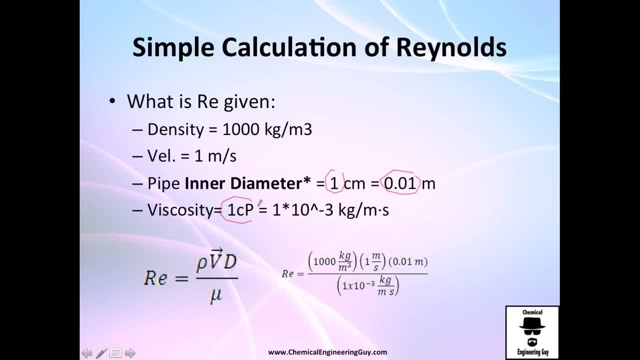 is point zero one meters, and one CP or centipoise is just one divided by thousand. so we plug numbers: one thousand here one meter, percent of here one zero one meter, and how much is that? we got the Reynolds number of ten thousand right here and it's actually 10 to the. 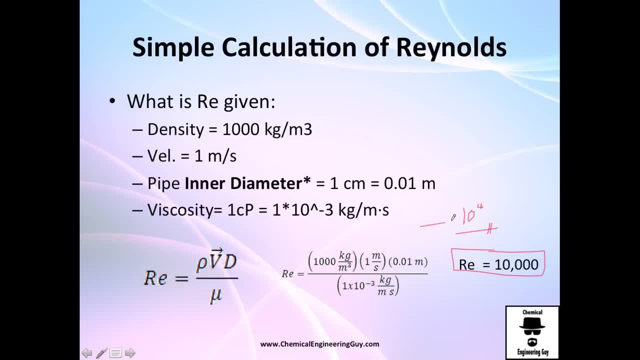 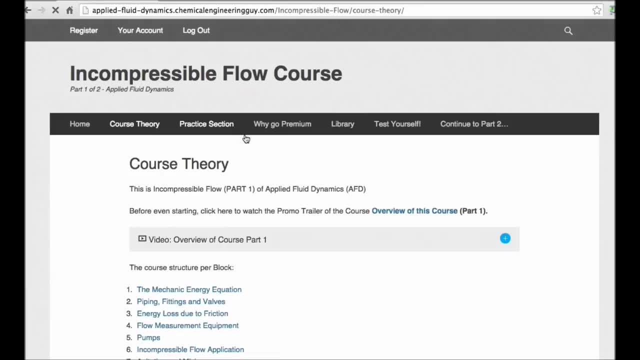 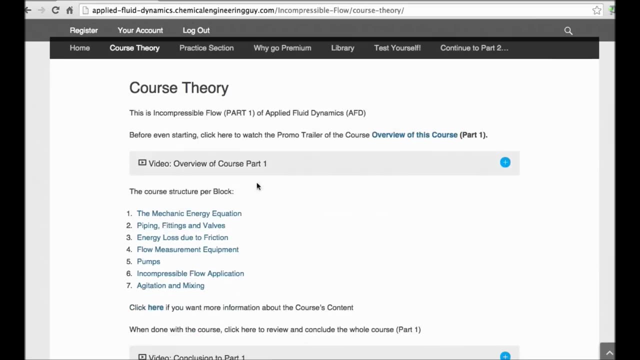 four power. you're going to see later that this is transient flow. it's not enough to be turbulent flow, so we want to avoid this right here. this was a free preview. you want to get access? go to my incompressible flow course. the link is in the description of the video. you will. 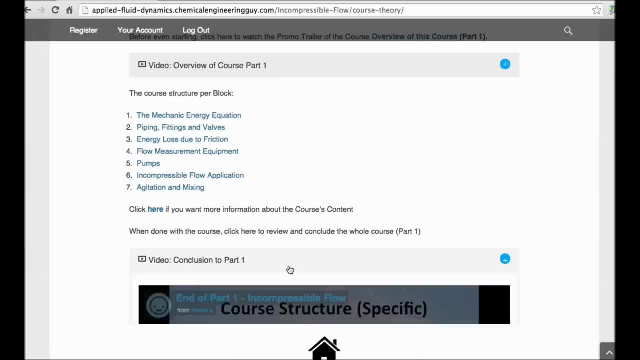 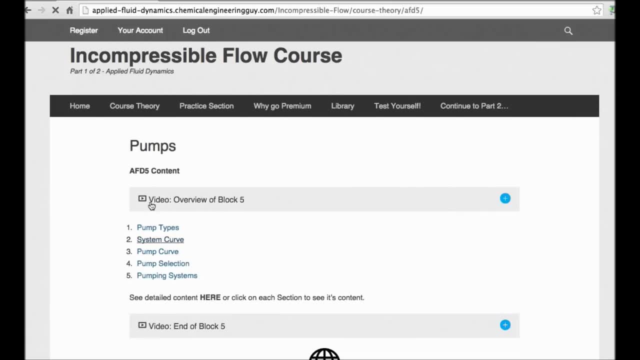 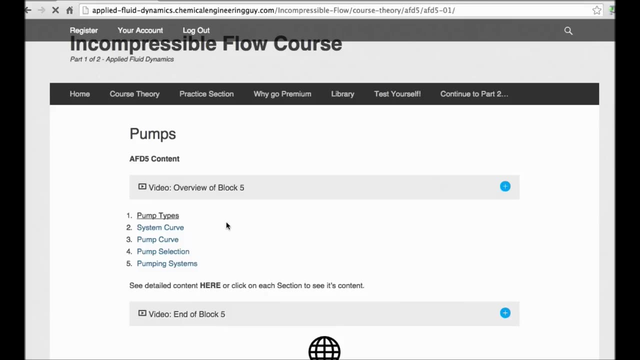 get all access. not only that, you get a very straightforward, user-friendly interface. so, instead of you were analyzing or studying pumps, you have it here: the pump block, then you have the sections. if you're, for example, studying the types of pumps, you can go here and you have all. 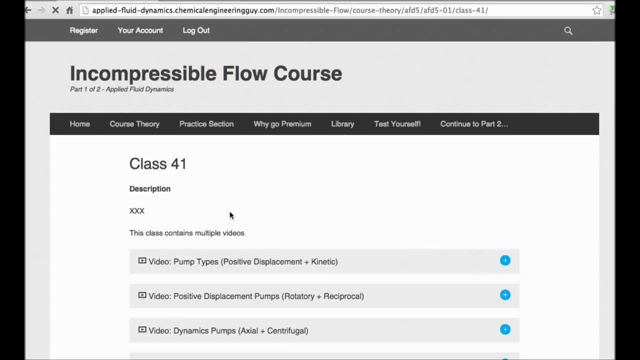 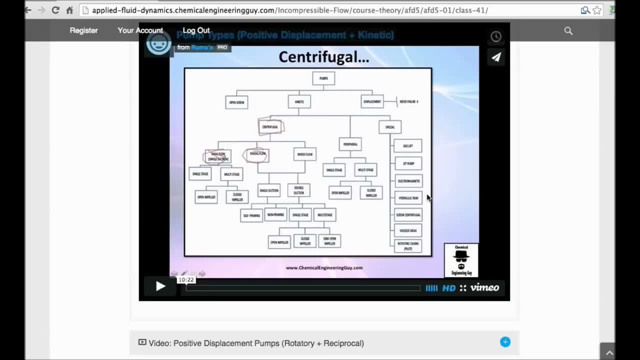 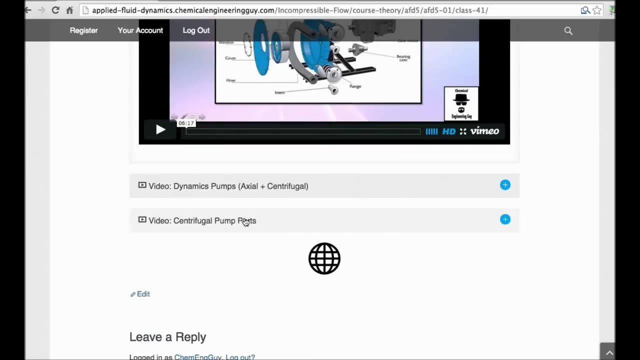 the classes right here, not to mention that you also have introduction and conclusion of every one of these. so, for instance, if you were studying positive displacement pumps, the video is right here. you were studying positive displacement pumps in rotatory and reciprocal. are also included here centrifugal pumps, which is a very important topic in this course. you have it right here.